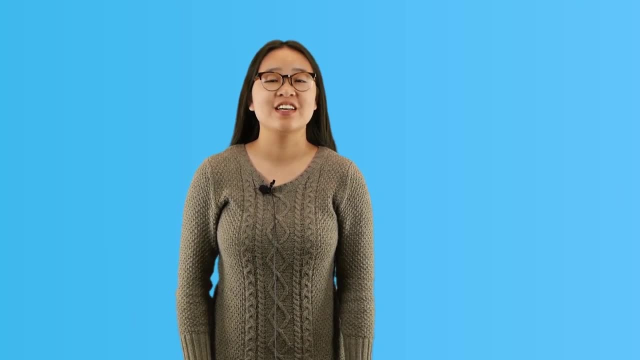 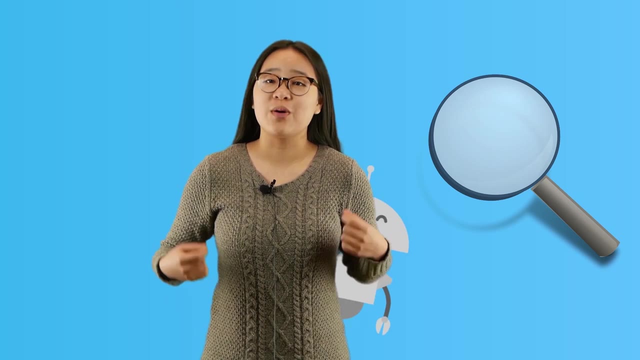 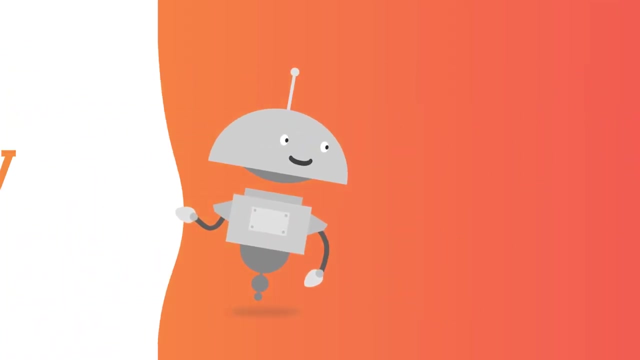 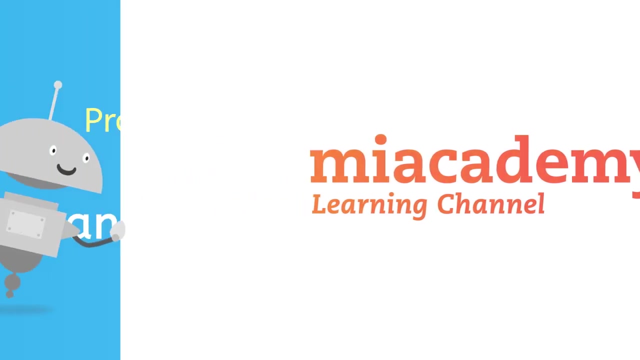 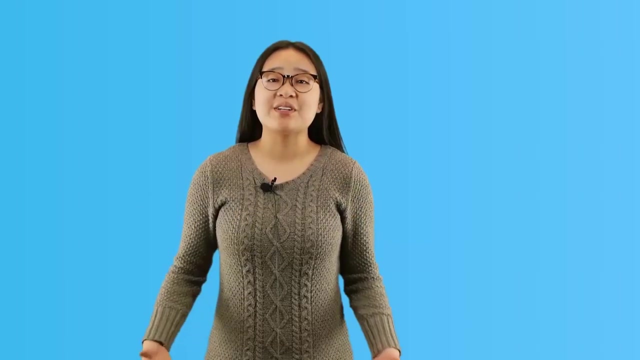 Hello and welcome to Problem Solving Strategies. 1. Looking for clues and key words. In this video you'll learn tricks for finding evidence or clues to help you solve word problems. How do you find the answers for a word problem When you're given a word problem to solve? 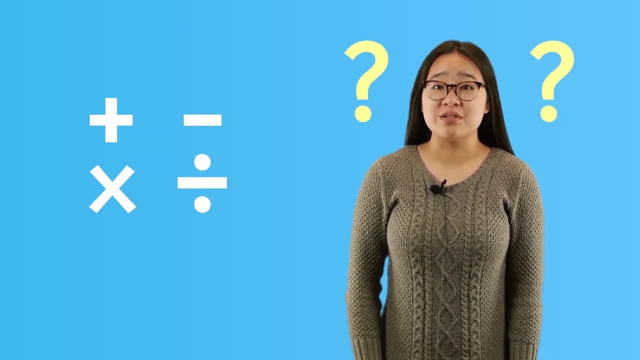 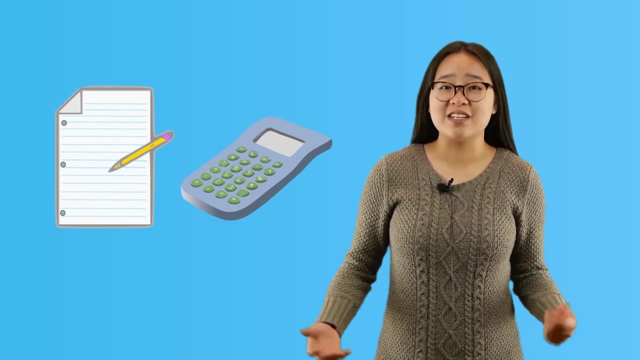 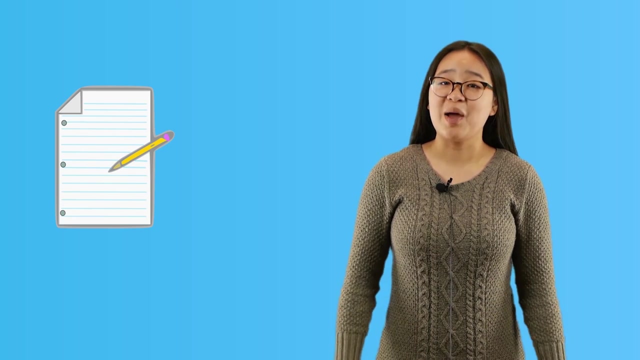 it can sometimes be confusing. How will you know what to do to find the answer? You know that you'll need to do some math calculation, but how do you know which one is correct? This is a common problem, but don't be afraid of word problems. I'm going to show. 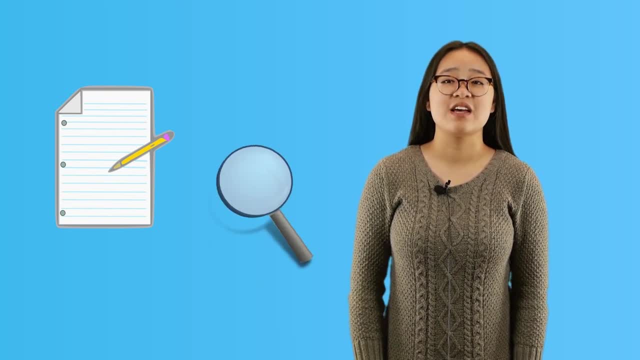 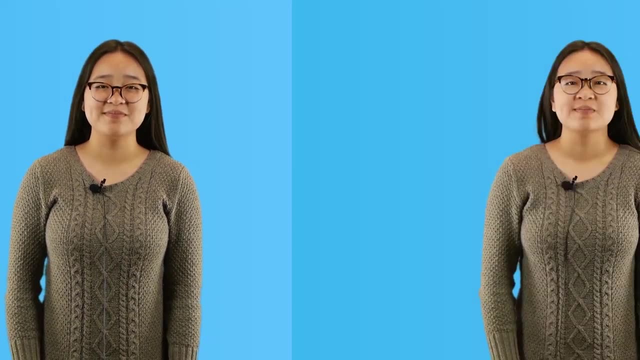 you some tricks, because every word problem gives us hints, no matter what the problem is, It's true. 1. What are some common clues? Let's look at them. Sometimes a word problem will ask you to add without using the word add. 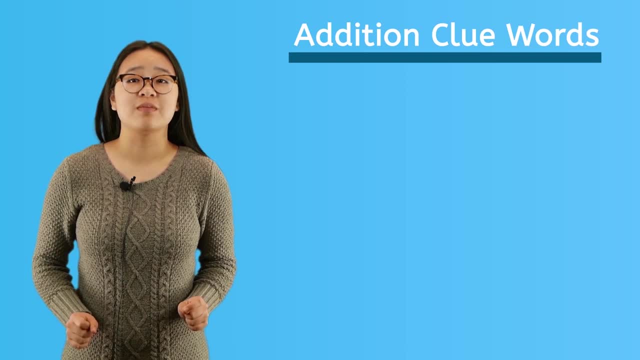 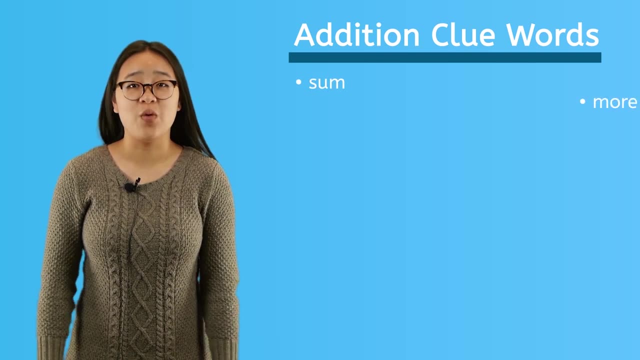 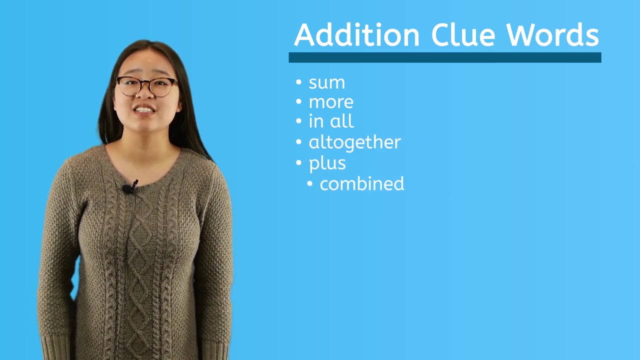 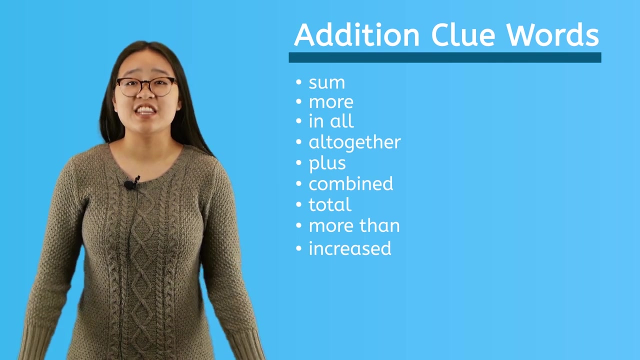 How will you know? There will be clues in the word problem that tell you you need to add. Those words are some more in all altogether plus combined, total more than increased. These words all mean the same as add. 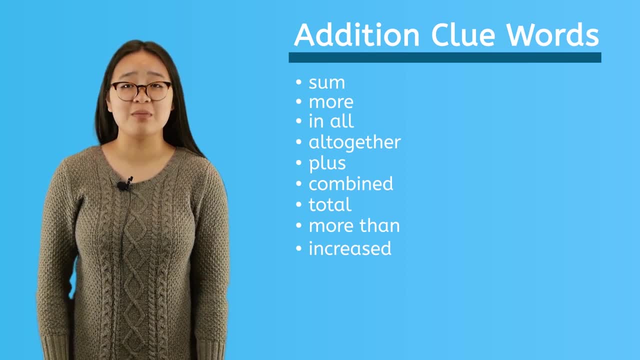 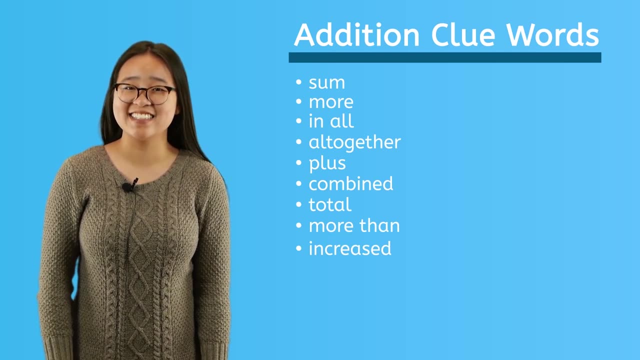 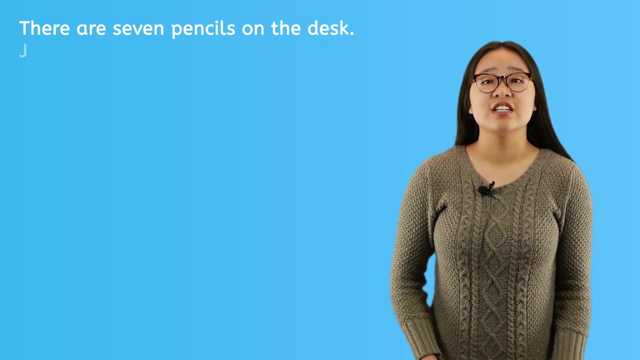 and they are clues that you will need to add to solve the problem. Let's look at an example where the word problem asks you to add without using the word add. Okay, here's a word problem. There are seven pencils on the desk. 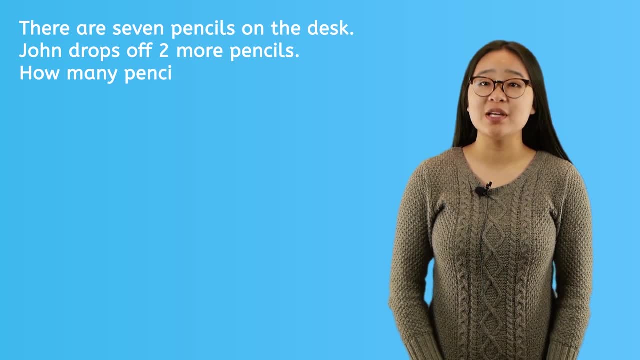 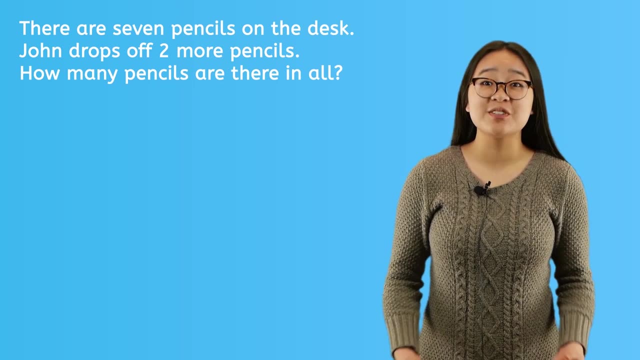 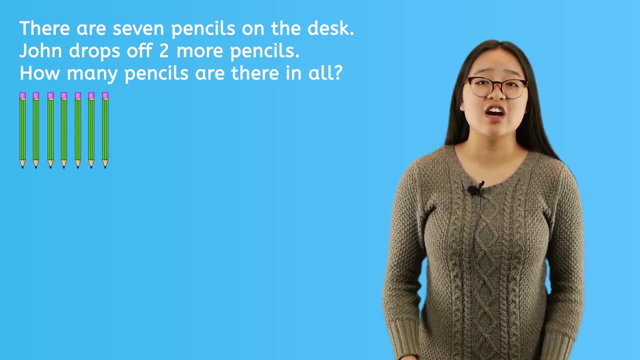 John drops off two more pencils. How many pencils are there in all? Now, how will we solve this problem? Let's look for clues or key words. We know that there are pencils on a desk and that John comes along and drops off more pencils. 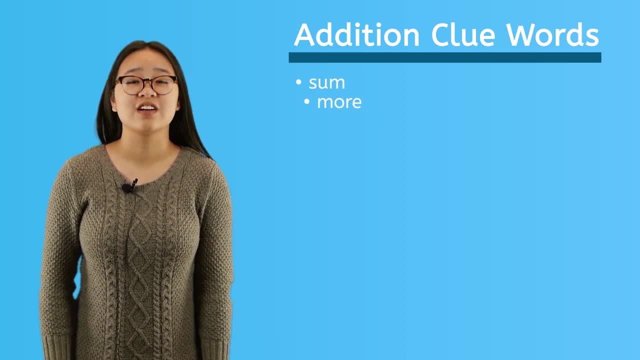 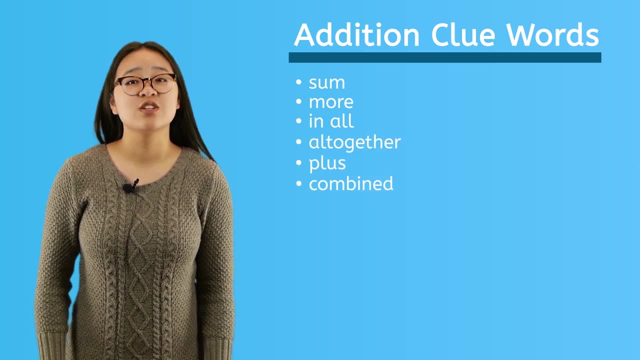 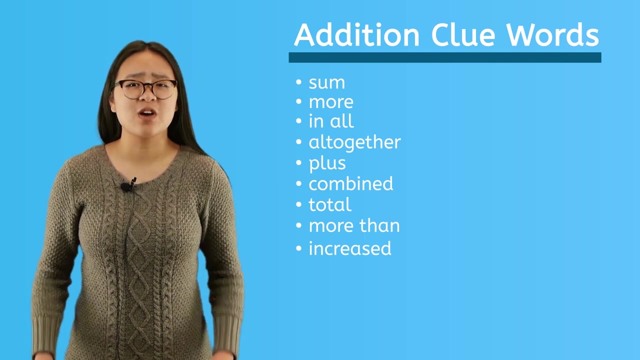 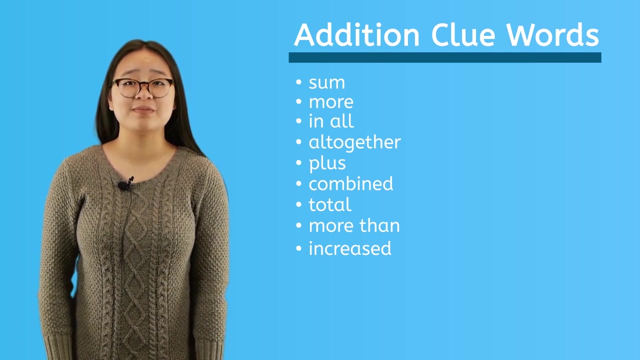 some more in all: all together, plus combined total, more than and more Increased. These words all mean the same as add, and they are clues that you will need to add to solve the problem. Let's look at an example where the word problem asks you to add without: 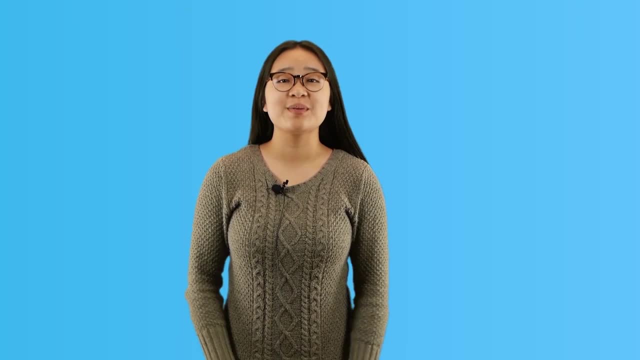 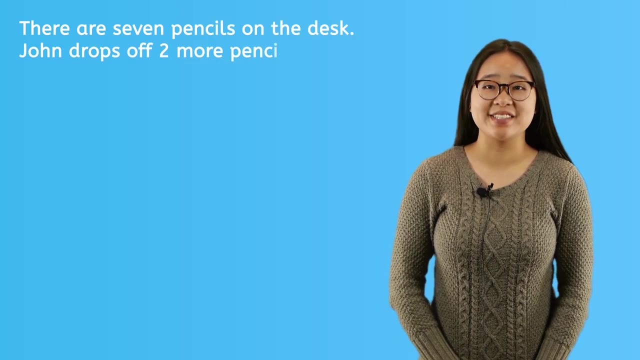 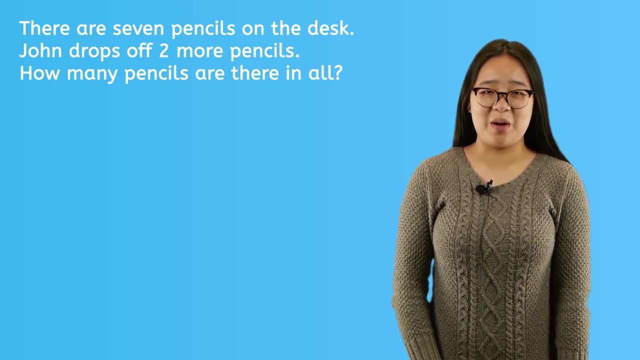 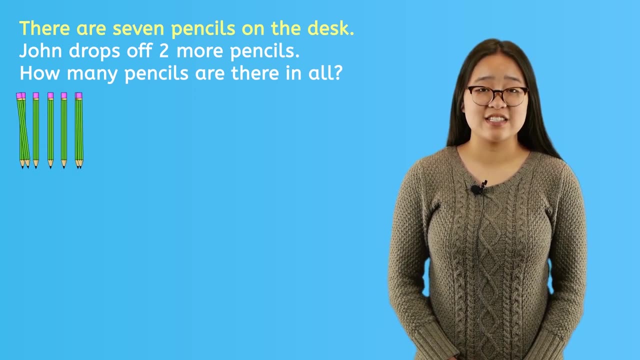 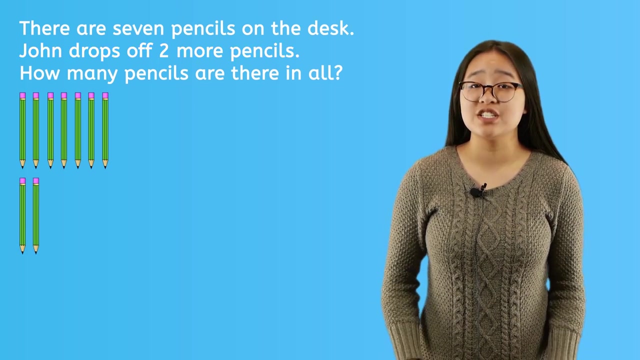 How many pencils are there in all of them? Now, how will we solve this problem? Let's look for clues or keywords. We know that there are pencils on a desk and that John comes along and drops off more pencils. The question asks: how many pencils are there in all? 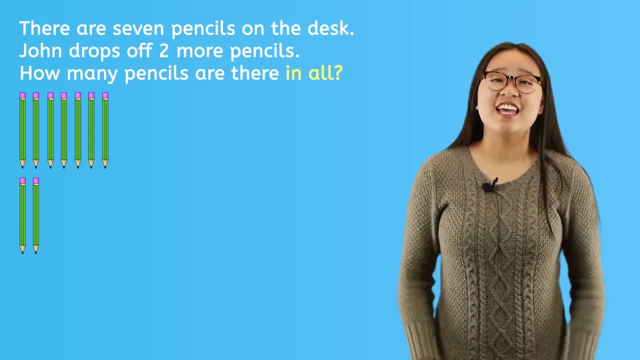 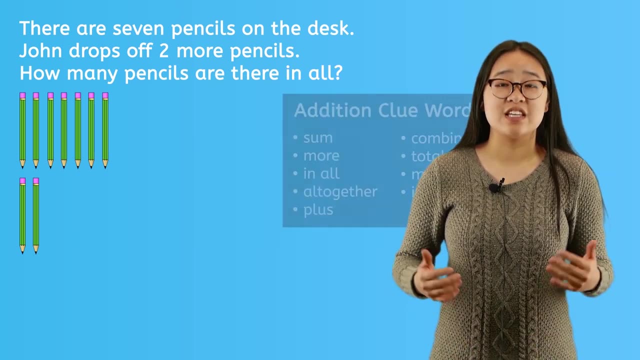 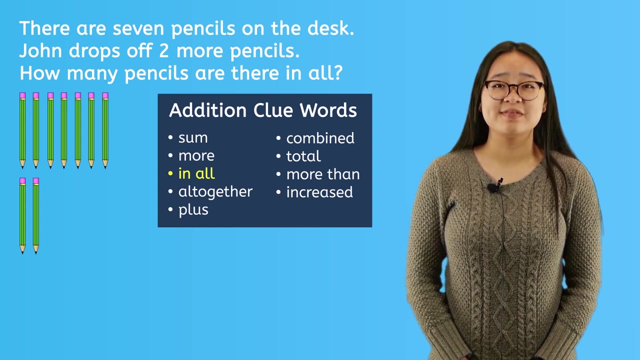 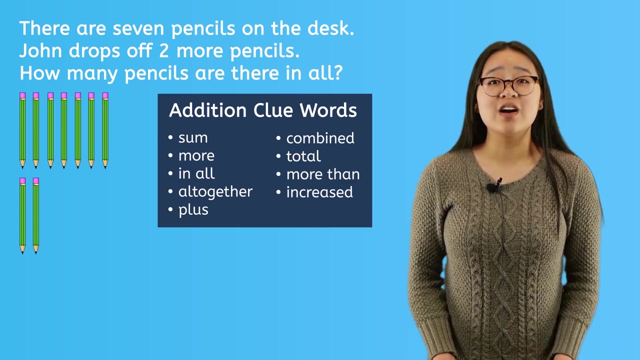 Do you see the clue in the question? Yes, you are right. In all is a clue You remembered from the word list given before. that in all is a clue to use addition in this problem: How many pencils in all Or how many pencils in total? 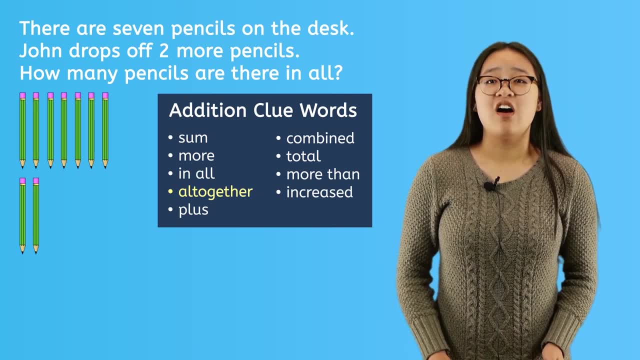 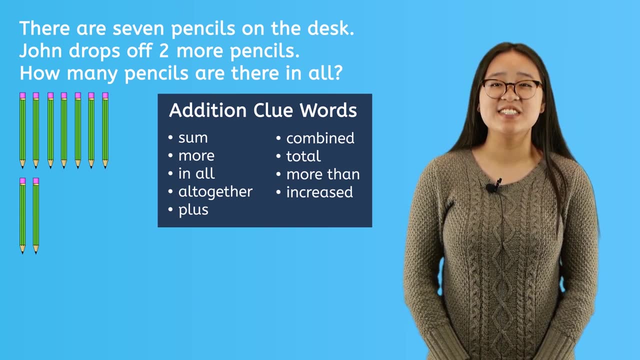 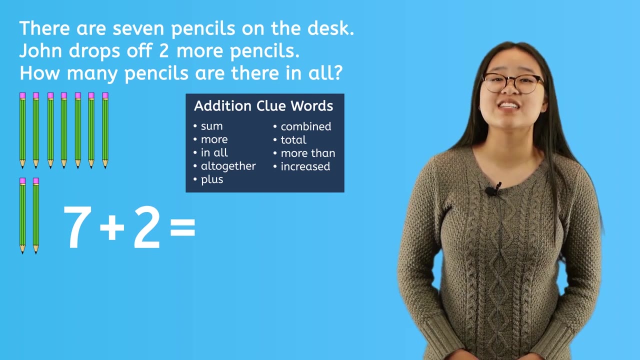 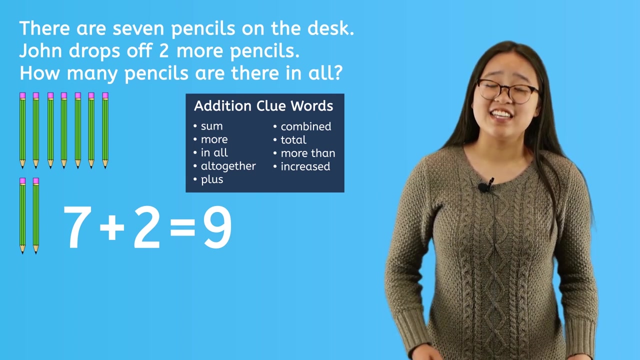 Or how many pencils all together. All of these mean the same thing And they all ask us to add. So 7 pencils plus 2 more pencils that John drops off equals 9 pencils. We've solved this problem by adding. The answer is 9 pencils in all. 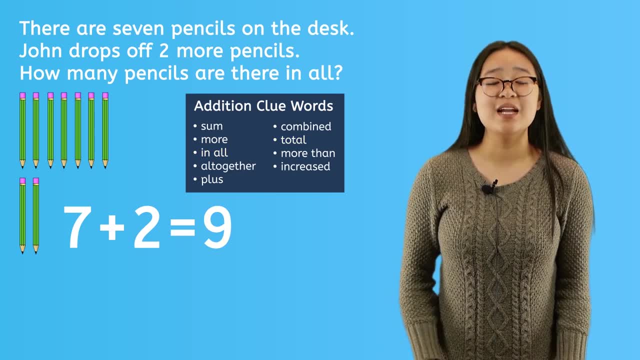 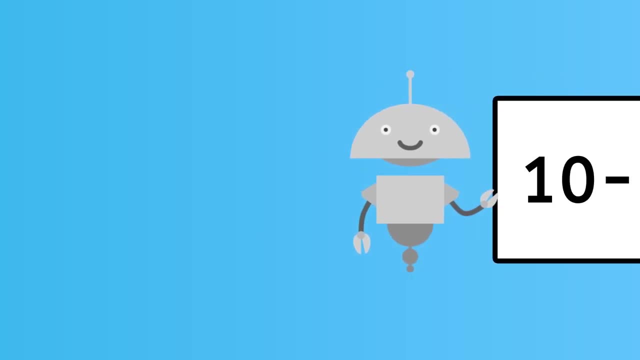 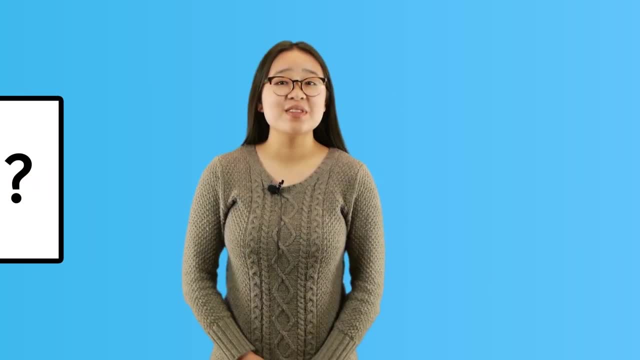 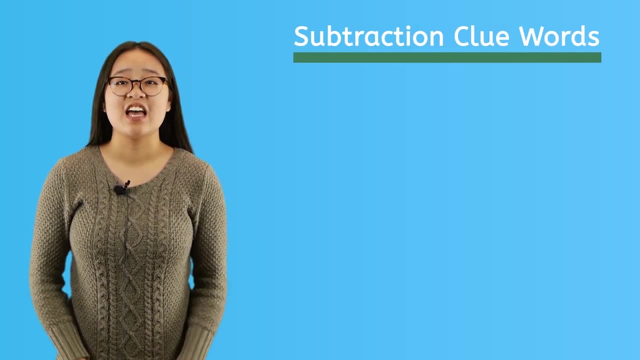 Subtract or minus. Subtract or minus. Subtract or minus minus? How will you know? Just like with addition, there will be clues in the word problem telling you that you need to subtract or minus. Those words are take away fewer than less than. 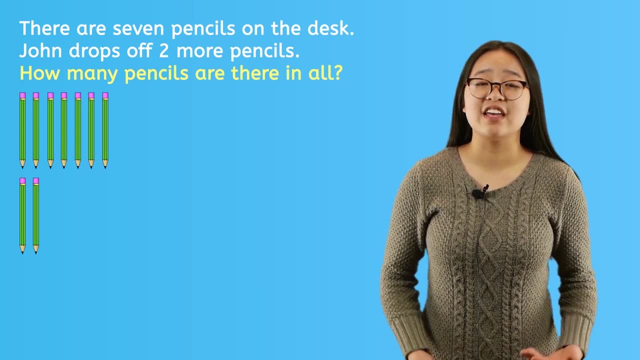 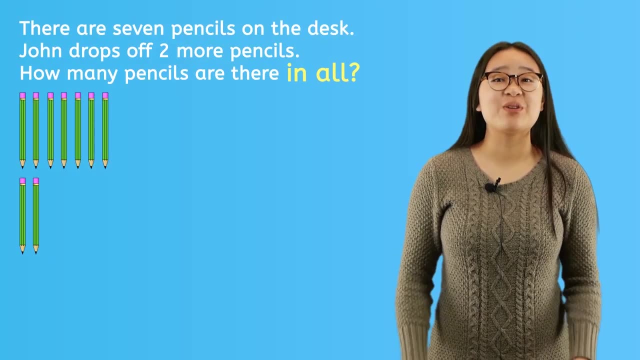 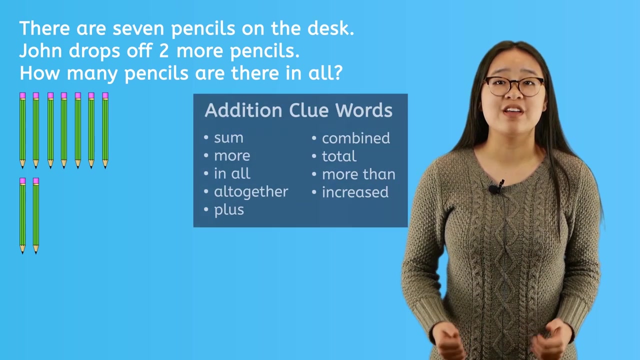 The question asks: how many pencils are there in all? Do you see the clue in the question? Yes, you are right. In all, All of these are clues You remember from the word list given before. that in all is a clue to use addition in this problem. 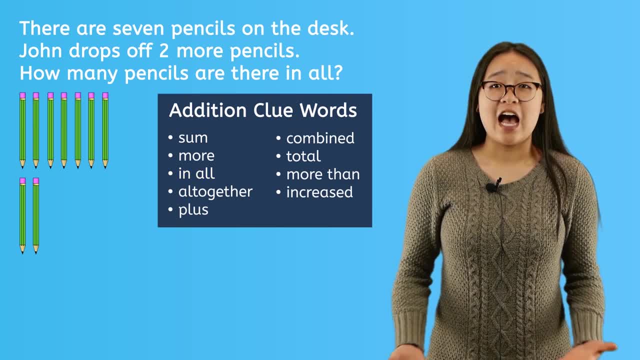 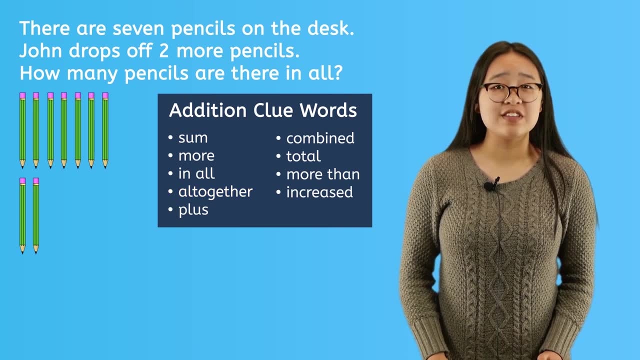 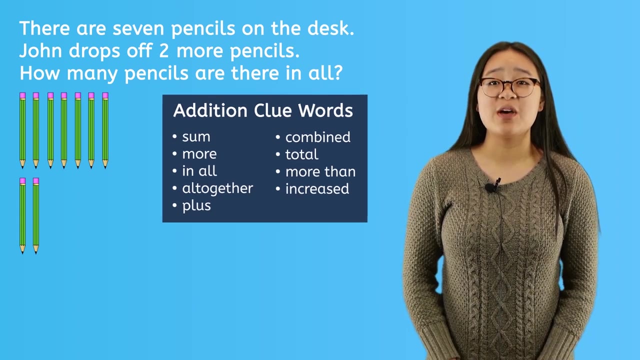 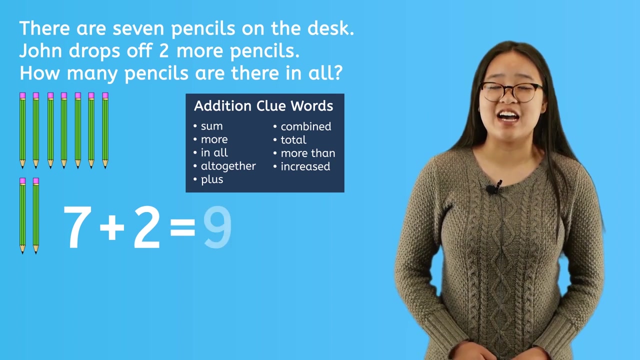 How many pencils in all, Or how many pencils in total, Or how many pencils altogether. All of these mean the same thing and they all ask us to add. So Seven pencils plus two more pencils that John dropped off equals nine pencils. 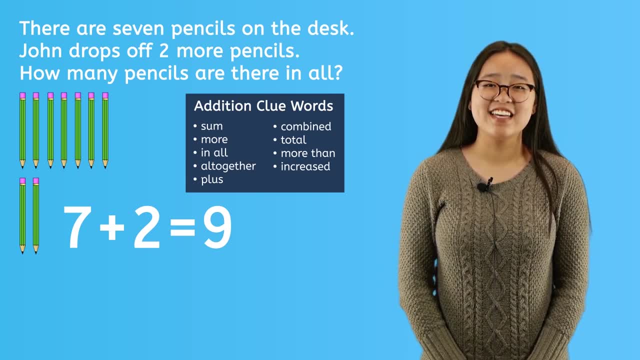 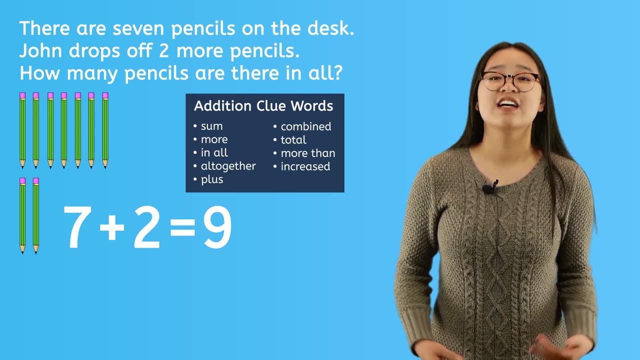 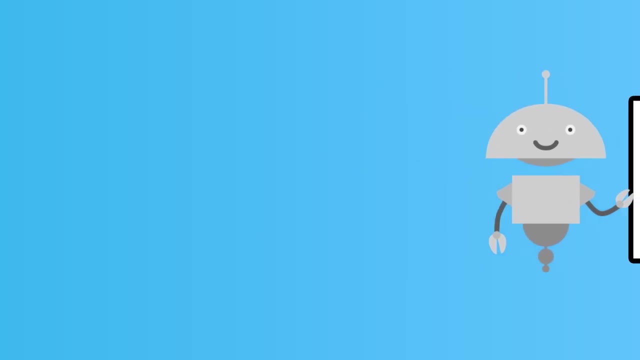 We've solved this problem by adding. The answer is nine pencils in all, or nine pencils in total or nine pencils altogether. Sometimes a word problem will ask you to subtract or minus without using the word subtract or minus. How will you know? 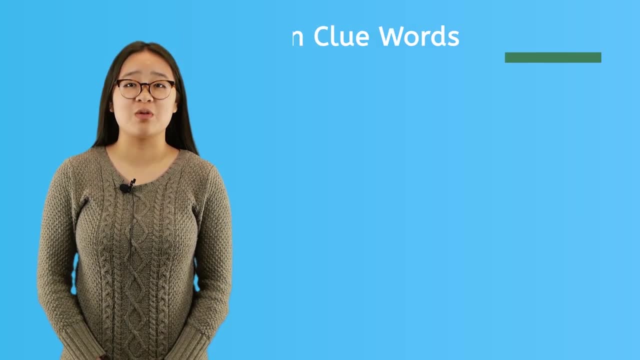 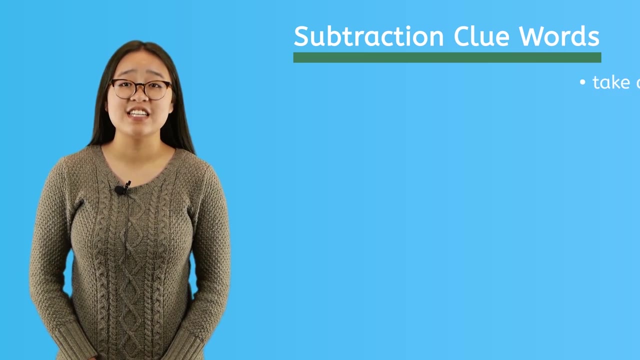 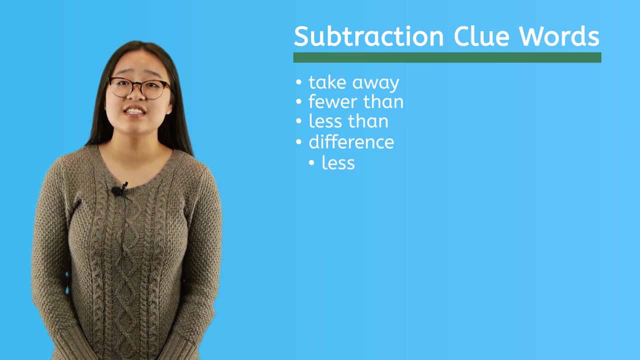 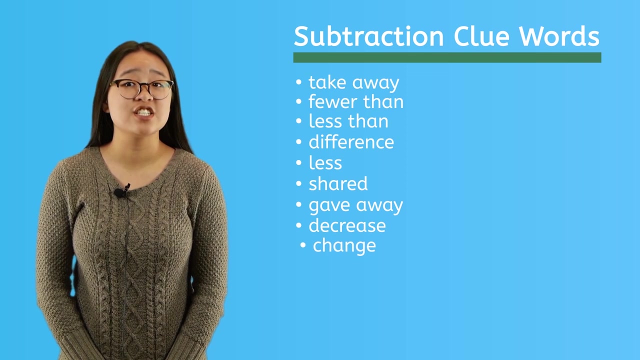 Just like with addition, there will be clues in the word problem telling you that you need to subtract or minus. Those words are: take away. fewer than less than difference, less shared. gave away, decrease, change left. 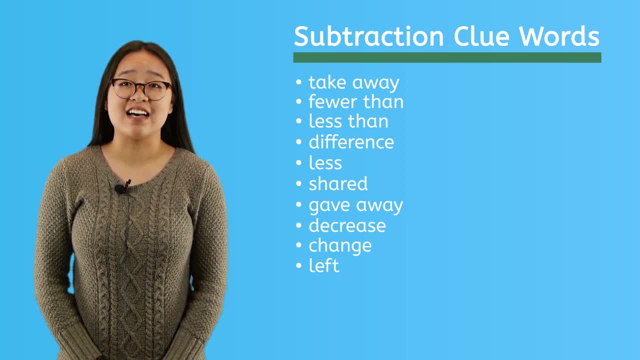 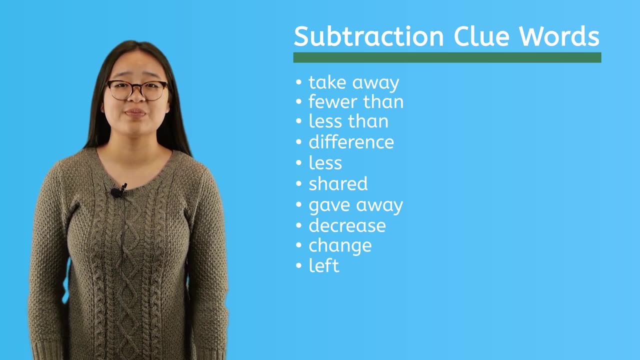 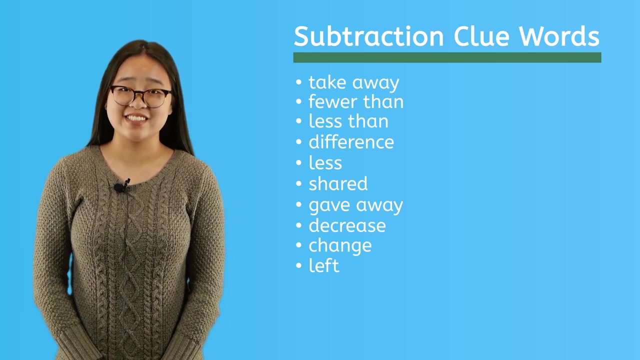 These words all mean the same as subtract or minus, and they are clues that you will need to subtract in order to solve the problem. Let's look at an example where the word problem asks you to subtract without using those words at all. Here's a word problem. 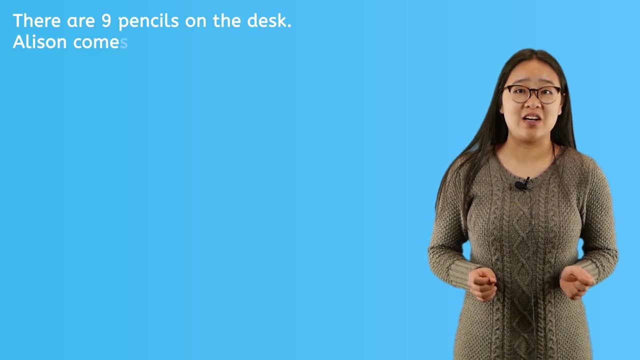 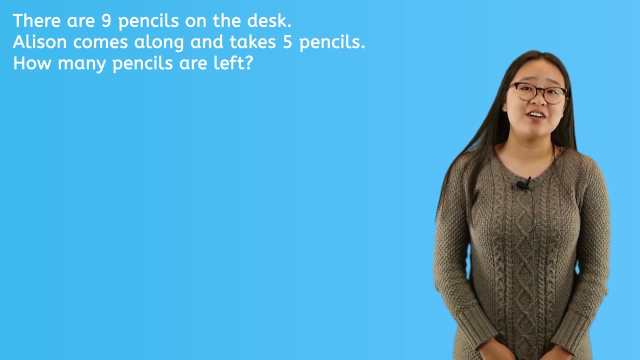 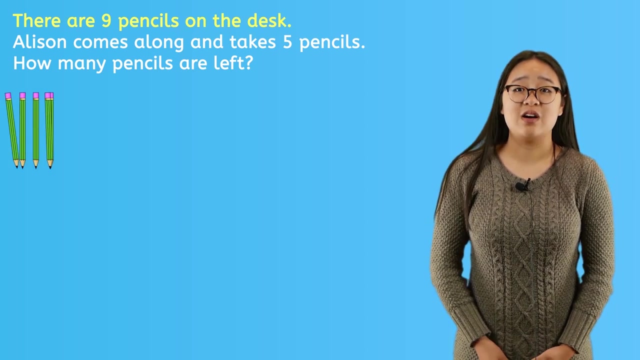 There are nine pencils on the desk. Allison comes along and takes five pencils. How many pencils are left? How will we solve this problem? Let's look for clues or key words. We know that there are nine pencils on a desk. We also know that Allison needed five of them, so she took them. 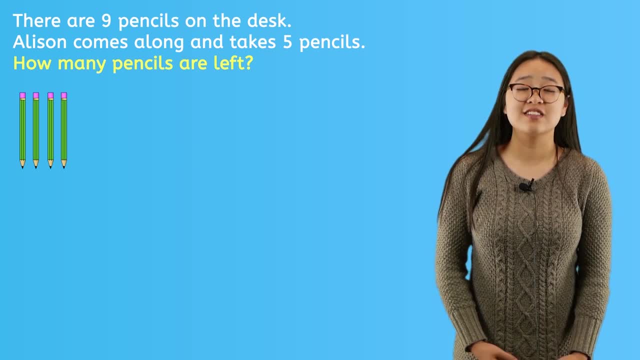 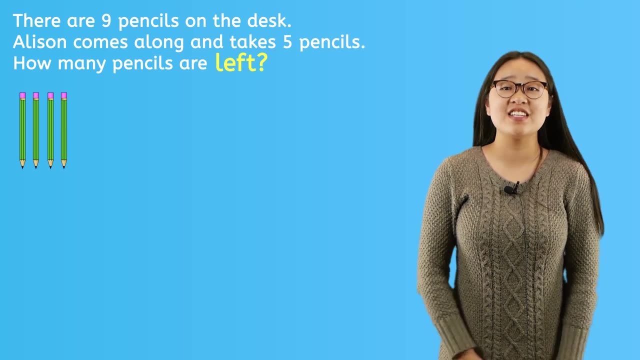 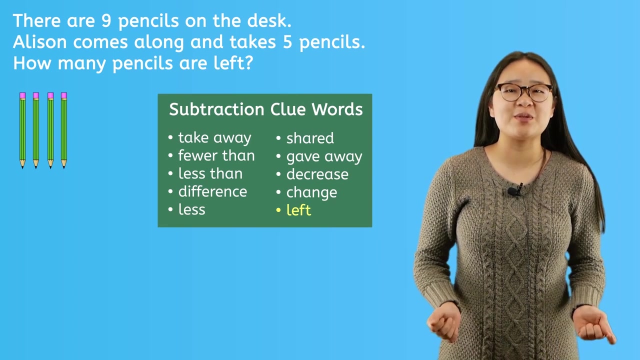 The question asks how many pencils are left. What is the clue in this question? Yes, you are right. again, Left is a clue. You remembered from the word list given before That left is a clue to use subtraction in this problem.